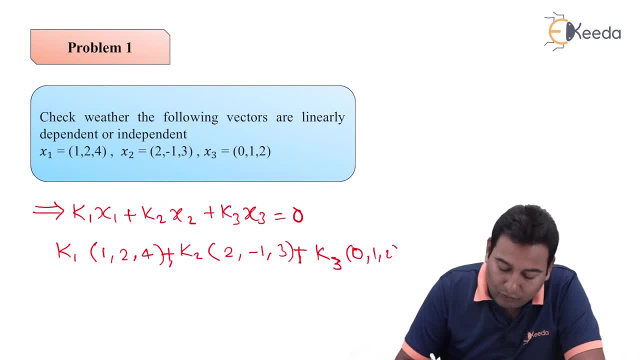 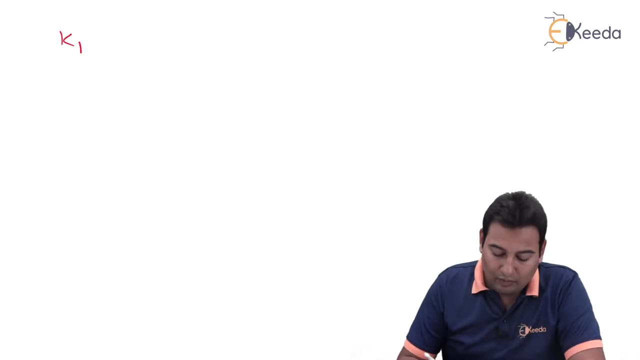 k3, x3, x3 is 0, 1 and 2 equal to 0.. Let us form the equation from this. Take the first term of all the vectors, that is, 1 multiplied with k1, this is 2, and this is 0 plus 2. k2 plus 0- k3- first term of all the vectors. 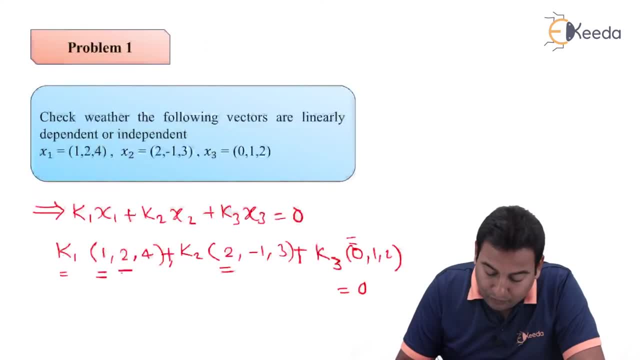 Next second term of all the vectors, That is 2 minus 1 and 1, that is 2 k1 minus k2 plus k3 equal to 0.. And the last is the last third term, that is 4, 3 and 2.. 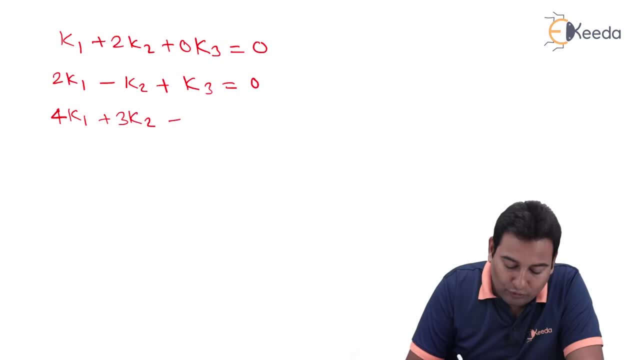 4 k1,, 3 k2,, 2 k3, equal to 0.. We got all the equation. Let us form matrix from it. Write it on the coefficients. here it will be 1,, 2, 0 in the first row, k1 coefficient. 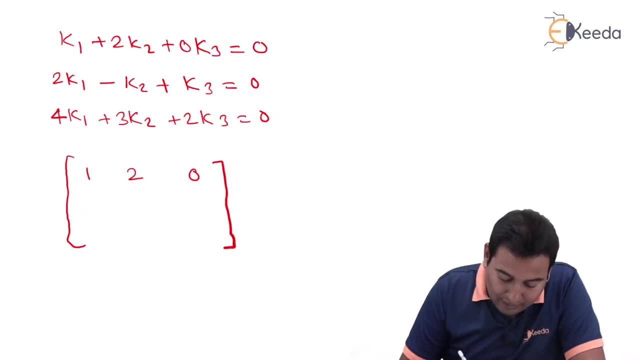 is 1, k2 coefficient is 2, k3 coefficient is 0.. Next it is 2, minus 1 and 1 and finally 4,, 3 and 2.. Here the unknowns are k1, k2, k3, and RHS is 0, 0 and 0. 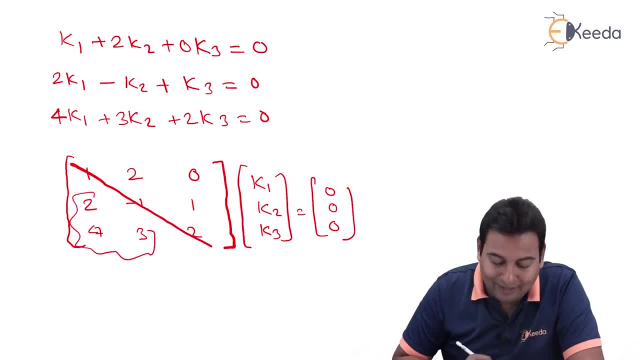 We need to convert the matrix into upper triangular matrix. That means we want to make these terms 0.. For that purpose, we need to perform the operations R2 minus 2R1 and R3 minus 4R1.. These are the basic operations. 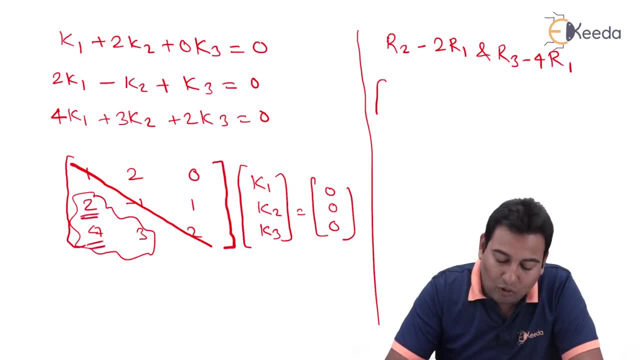 I want to make this 2 and this 4, 0.. Let's apply these operations Here, friends. R2 and R3 will remain same. only R1, R1 will remain same. R2 and R3 will change. So let me write it down quickly. which is same, that is R1. 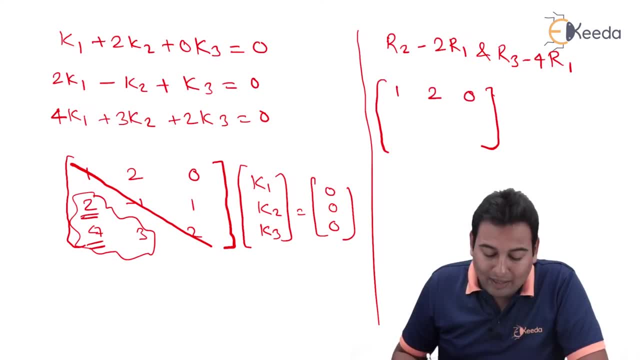 Let's check what will be the difference: R2 minus 2R1.. This will be 0.. This is minus 3, because R1 is multiplied to minus 2, and here it is 2.. 2 into minus 2 is minus 4 and minus 1, that is minus 5.. 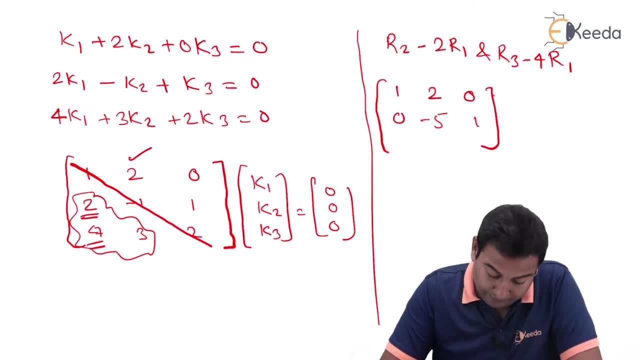 Here it is 1.. Next, R3 minus 4R1.. This is 0.. Minus 4 into 2 is minus 8, minus 8 plus 3 is minus 5, and this is 2.. The unknowns are k1, k2, k3, k3 and 0. 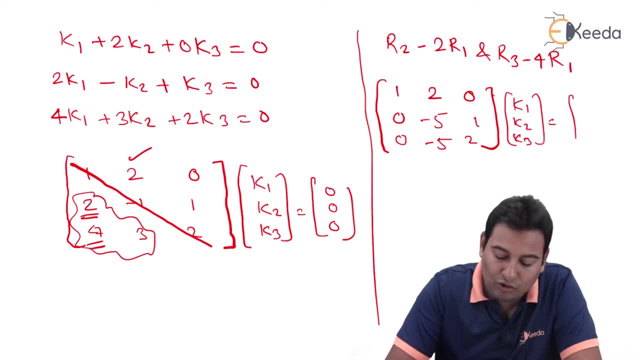 We are not yet done. We need to convert it into upper triangular matrix. That means still, we are left with: one value is to be made 0. This will be 0 with the help of this value. Therefore, it will be R3 minus R2.. 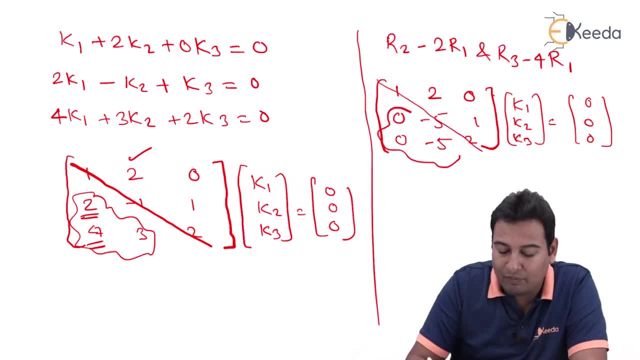 In R3 minus R2, only R3 will change, Only the first term will change. R1 and R2 will remain same. That I am going to write it down: 1, 2, 0.. 0 minus 4R1.. 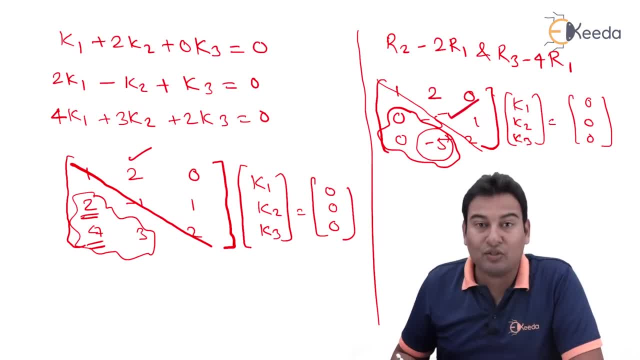 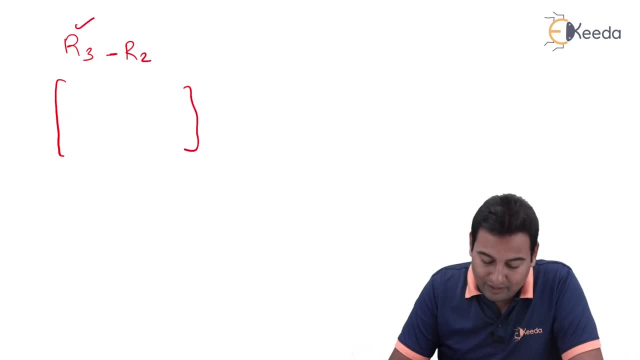 Only the first term will change: R1 and R2 will remain same. That I am going to write it down: 1, 2, 0.. 0 minus 5N1 and the last row will be 0, 0.. 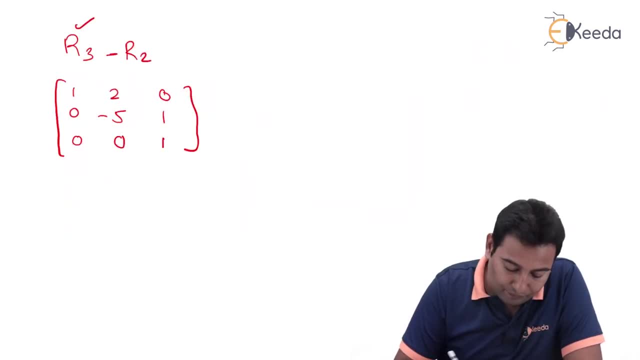 R3 minus R2.. That is 1. K1, k2, k3, which is equal to 0, 0, 0.. this was our aim and we converted the matrix into upper triangular matrix. what next if we are done? 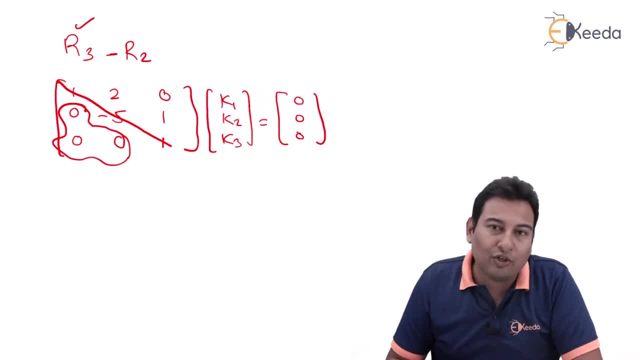 with that, let's move on to the next step. let's form the equation: first row: multiply to the first column in the first row we have 1, 2, 0. that will multiply to x 1, x 2 and x 3. that is a k, 1 k, 1 k. 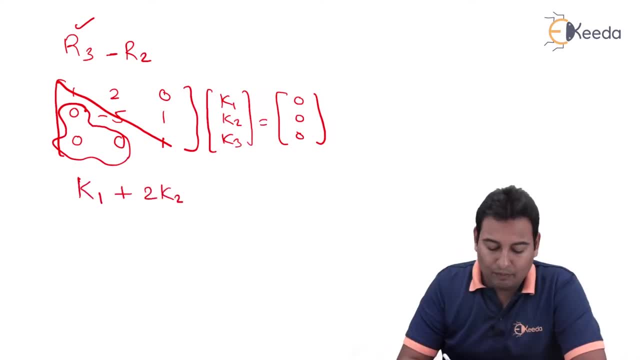 2 k 3 plus 2 k 2 plus 0 k 3- equal to 0. next next row is 0 minus 5 and 1. that will multiply to k 1, k 2, k 3, 0 k 1 means nothing minus 5. k 2 plus k 3- equal to 0. and from the last row we do have 0 0 1. 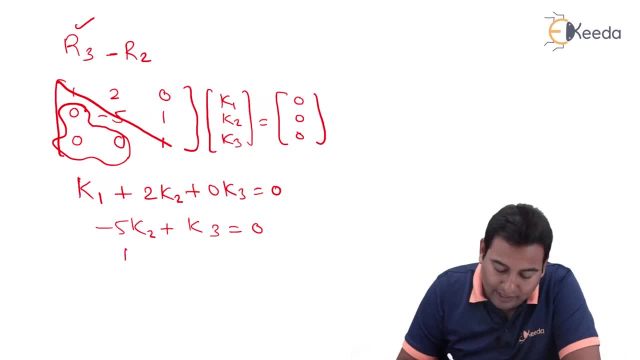 0, k 1, 0, k 2 and k 3. that means only k 3, k 3 equal to 0: 0.. If you put k3 equal to 0 in equation number 2, then you will get minus 5k2 equal to 0. that.